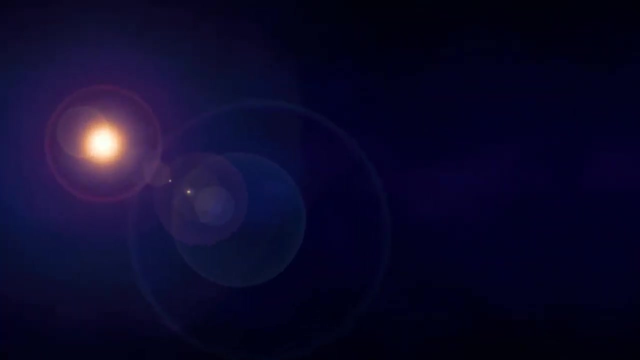 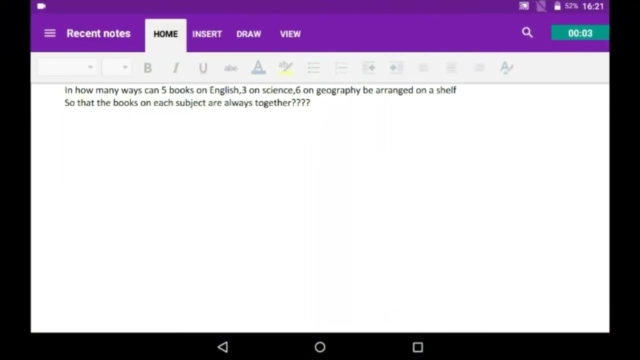 In how many ways can five books on English, three on science, six on geography be arranged on a shelf so that the books on each subject are always together? You have to arrange the books in such a way the same books on category, that is, English category books, should be together. 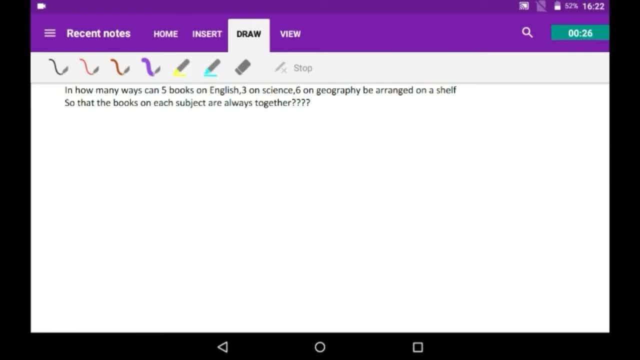 and science category books to be together and geography books should be together. That is, consider, if it is the shelf three partition for three subjects. I will place English here, science here and geography here. That is, I have to place the five books here, all the five books: one, two, three, four and five English books and 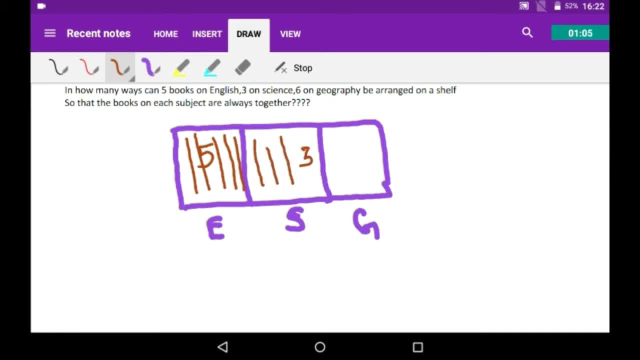 three science books: one, two and three, That is, three science books and six geography books. I have to place it this way. So they are asking you: in how many ways can you arrange it this way? So you have placed all the English books in a single rack, So you can consider it as a single unit, one unit, Right The same, like you can think this also as a one unit And you can consider geography also as a one unit. 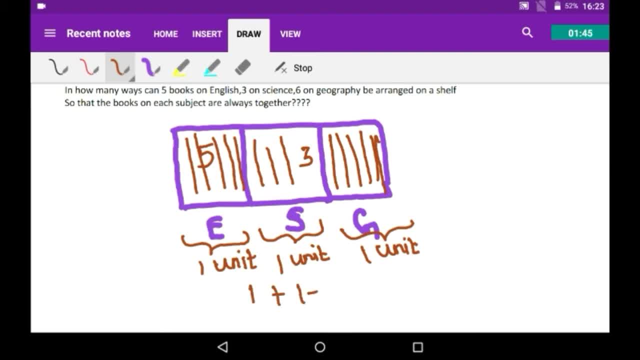 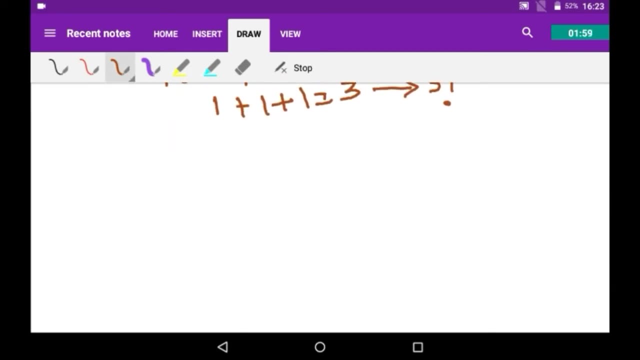 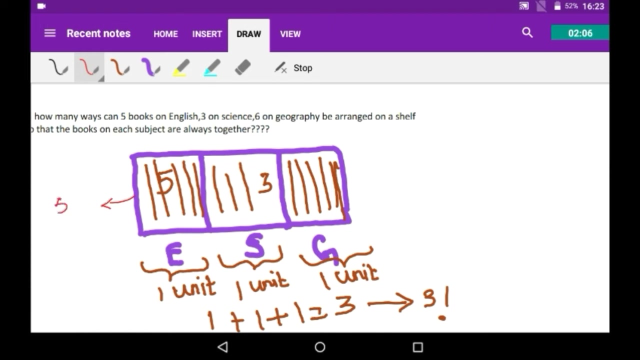 So total number of units is equal to 1 plus 1 plus 1 is equal to 3.. Right, So this can be placed in 3 factorial ways, Am I right? Next thing: the 5 English books can be placed in this. 5 English books can be placed in 5 factorial ways, Correct. 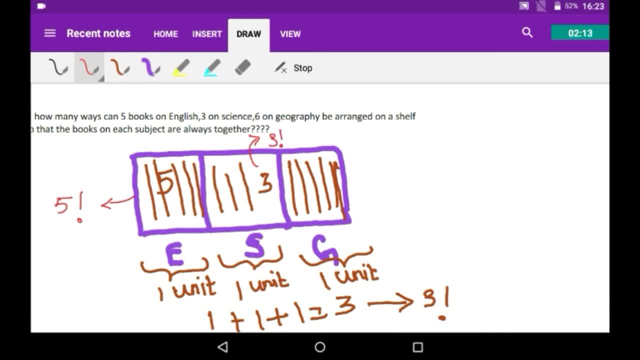 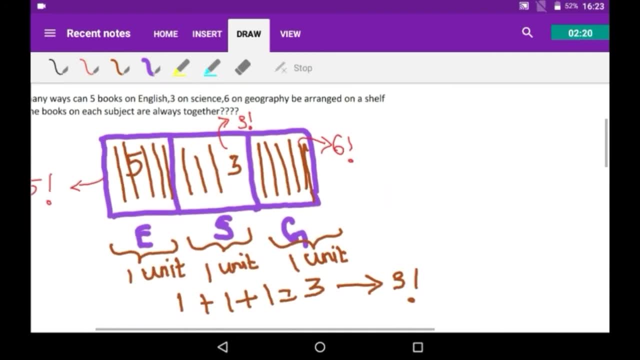 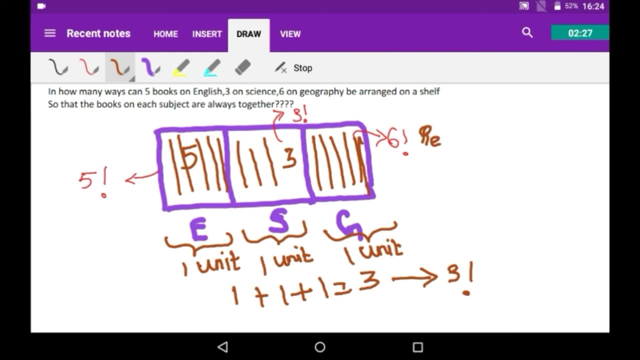 And 3 English books can be placed in 3 factorial ways And 6 geography books can be placed in 6 factorial ways. Correct, So the required number of ways will be required number of ways is equal to this 3 factorial into.